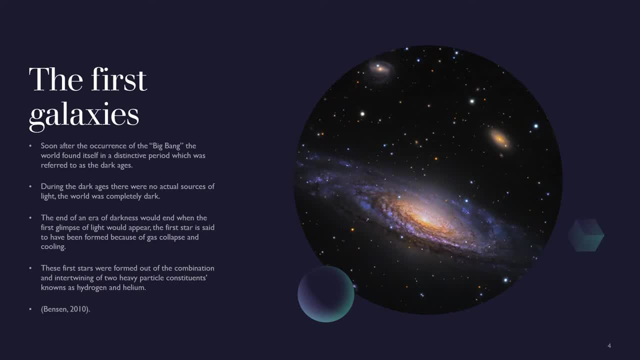 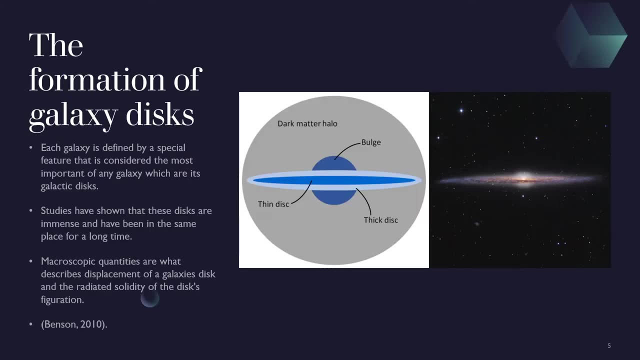 which are called constituents, which are known as Hydrogen and Helium. The formation of galaxy disks: Each galaxy is defined by a special feature that is considered the most important of any galaxy, which are its galaxy disks. Studies have shown that these disks are immense and have been in the same place for a very long time. 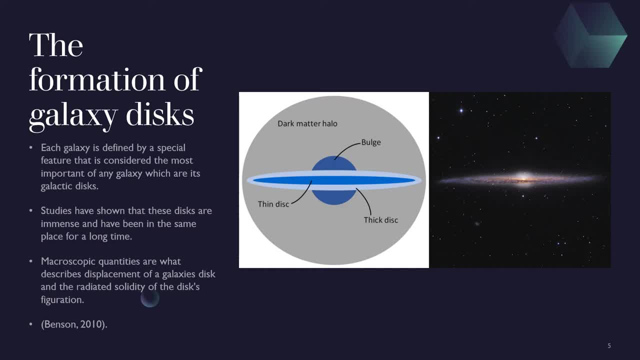 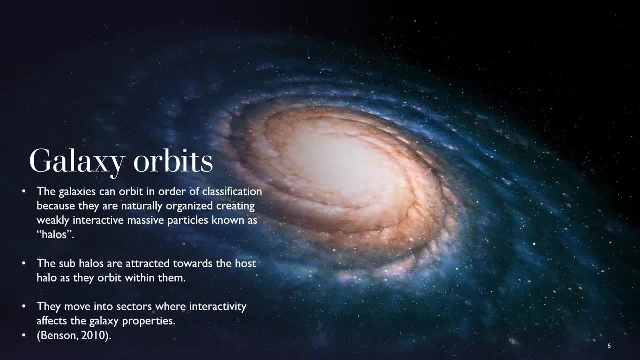 Microscopic quantities are what describe the displacement of galaxy disks and the radiated solidity of the disk's figuration. Galaxy orbits. Galaxies can orbit in order of classification because they are naturally organized, creating weakly interactive massive particles which are known as halos. 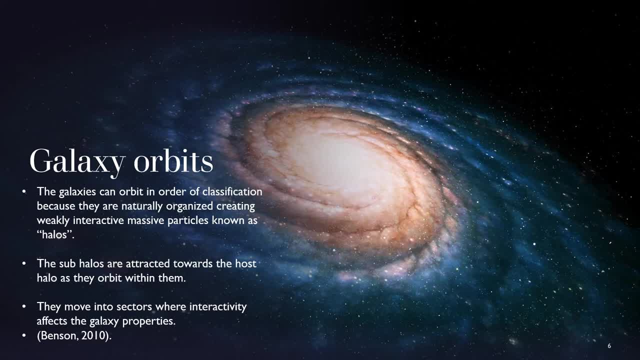